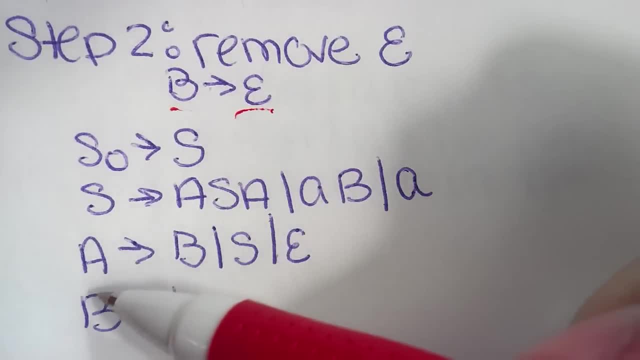 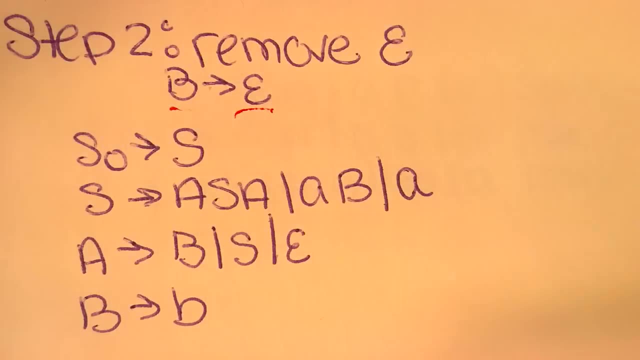 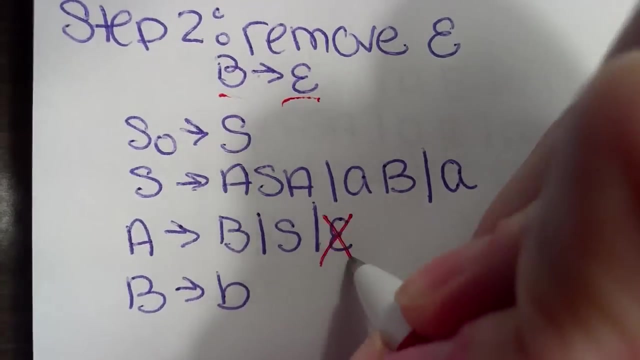 to asa or av or terminal a. We have our a points to b, s or epsilon And we have b pointing to terminal b by itself. Next step is to remove a points to epsilon. So, as you can see, here we cross off the epsilon again And then we find each instance of a where we need to. 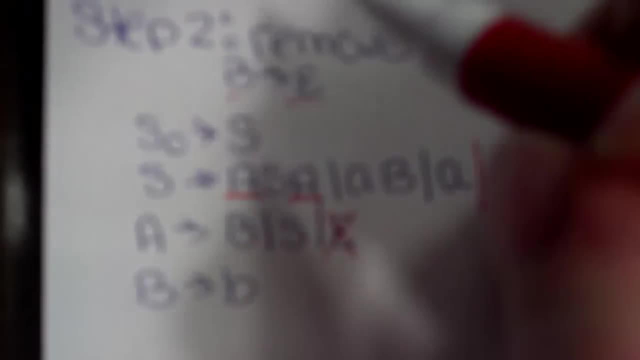 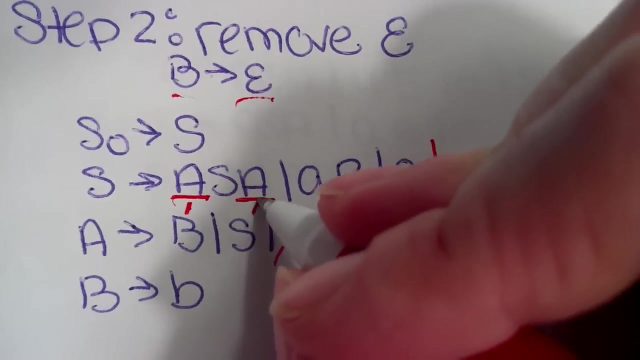 pretend it's an epsilon. So, as you can see, we first have to take into account if this a is an epsilon, So that would give us an sa. Then we can take into account if this a were an epsilon, which would give us an as, And then we have to take into account. 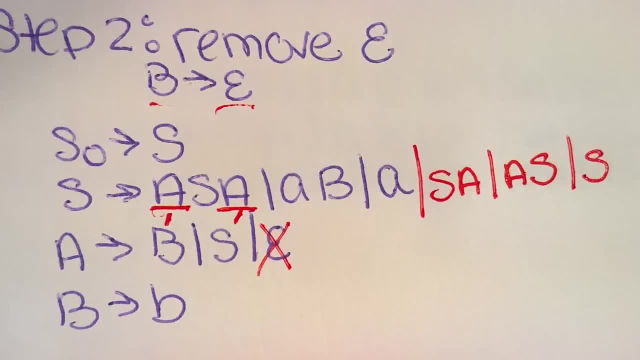 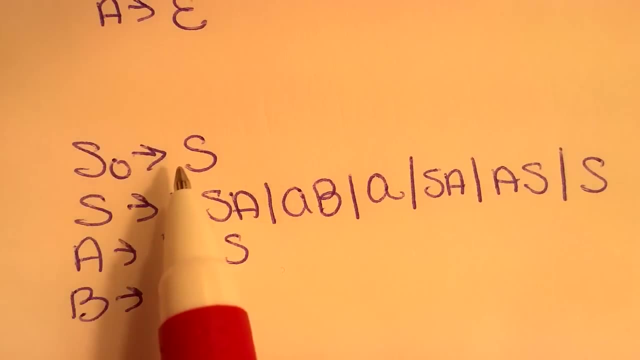 if both are epsilon, which would just give us s. So our new grammar looks like such. So we still have our first initial state, and now we have removed all of our epsilons. The second rule, or the second step to do now is to remove all of our unit rules. So first, 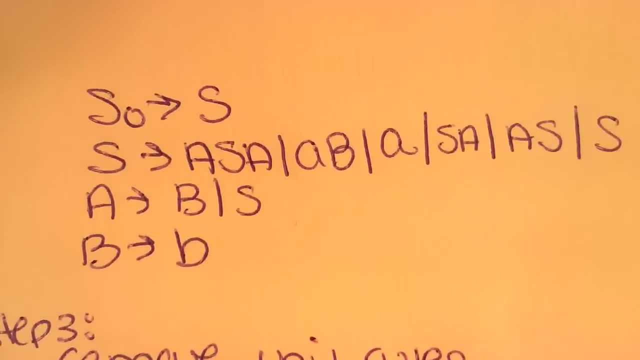 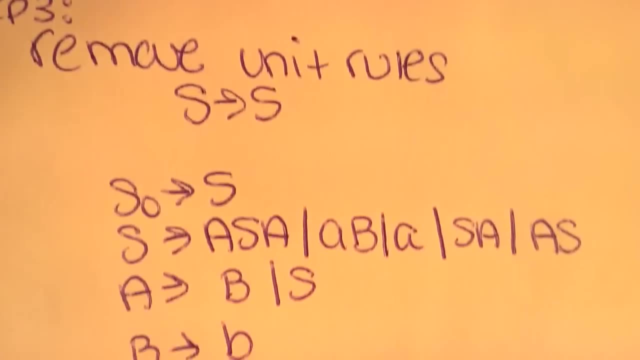 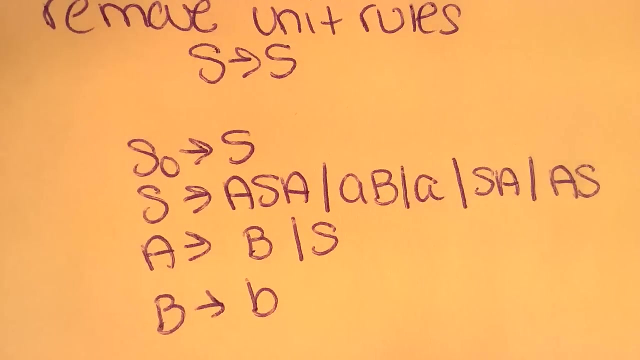 we're going to remove s points to s, which is the simplest, Since s refers to itself. we can just cross s off And our new equation looks like: so 2, 2, 2 rule is to remove s-naught points to s, which is just as simple, since s-naught points to. 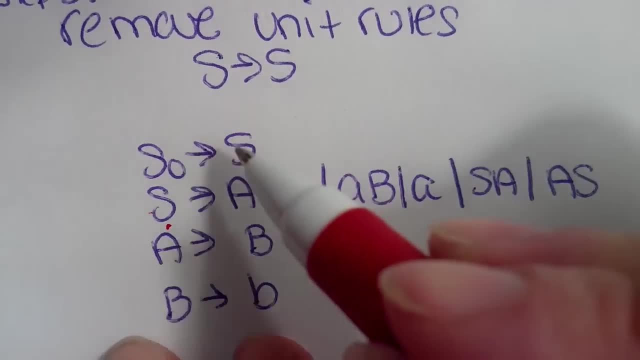 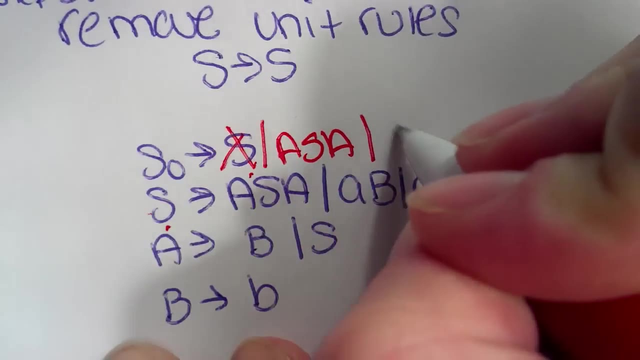 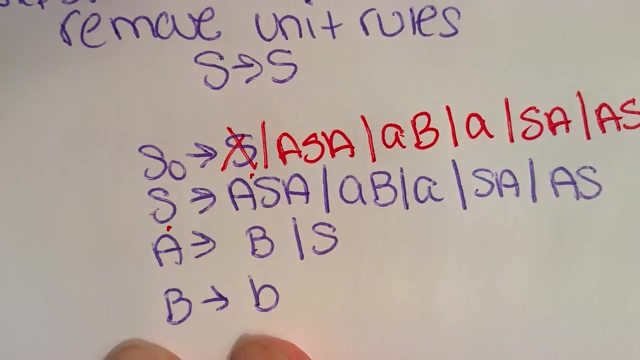 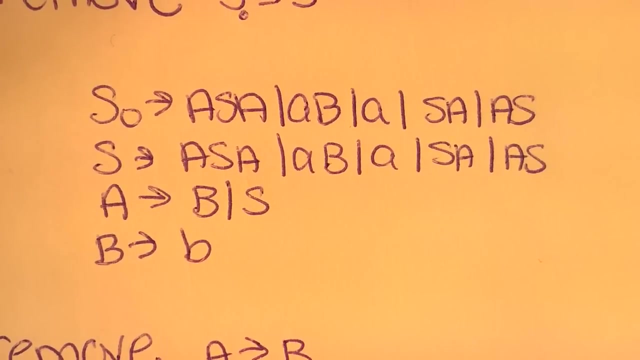 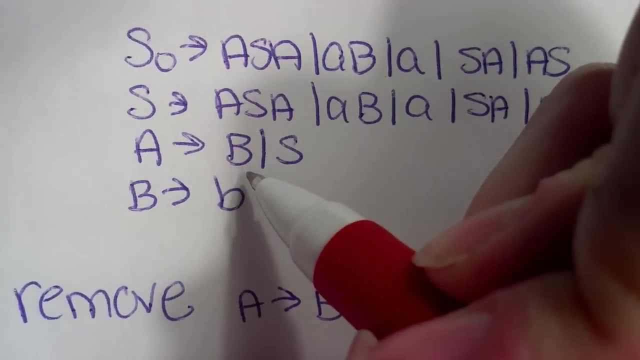 s and we know what s is. we just replace everything in s-naught with s, So we would cross off s and put in asa or ab or a or sa or as That would then make our new equation look like. so Now we need to remove a-points-to-b. So we look at b here and we see that b is only. 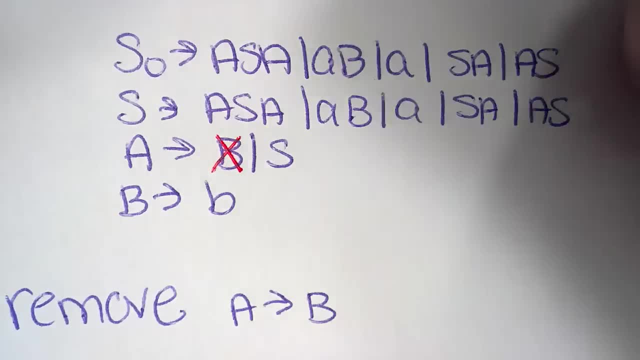 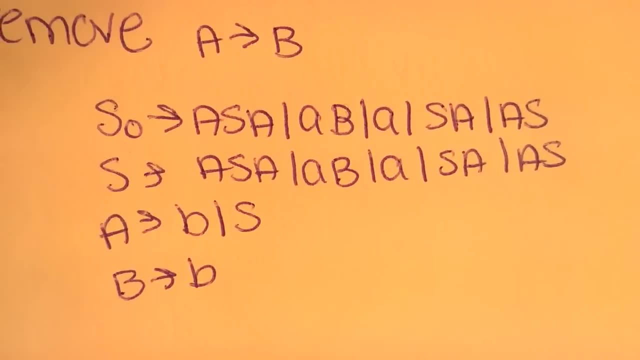 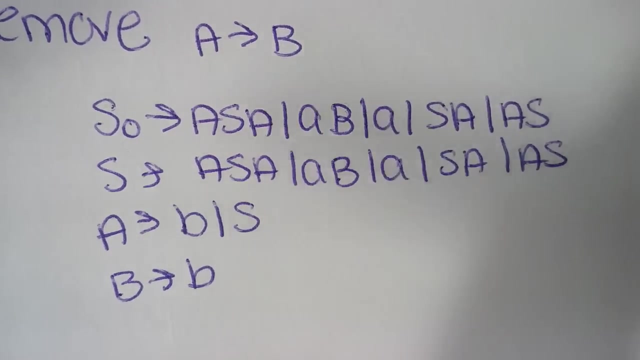 lowercase b, so we can just cross off our big B and replace it with ab, and now that's finished. Our new equation is like: so Now a-is only pointing to lowercase b, and uppercase s Next step is to pass any wrong entered information into the upper formula we just drew, and". 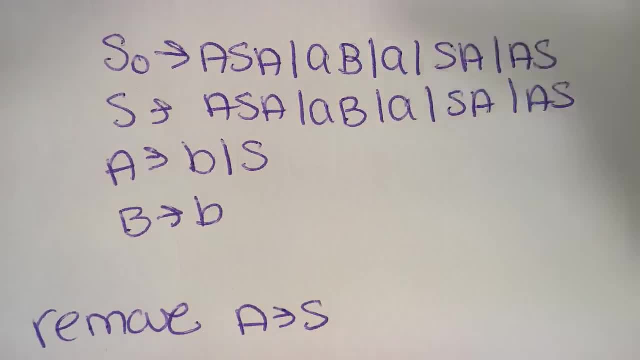 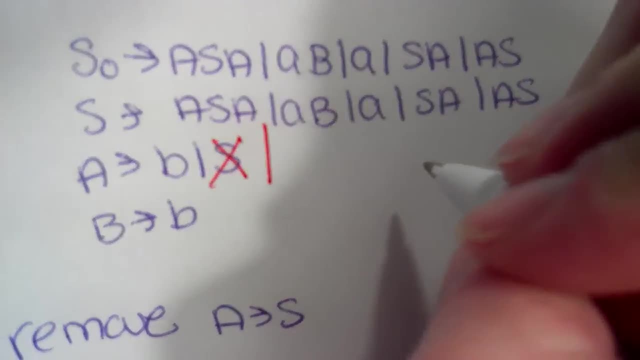 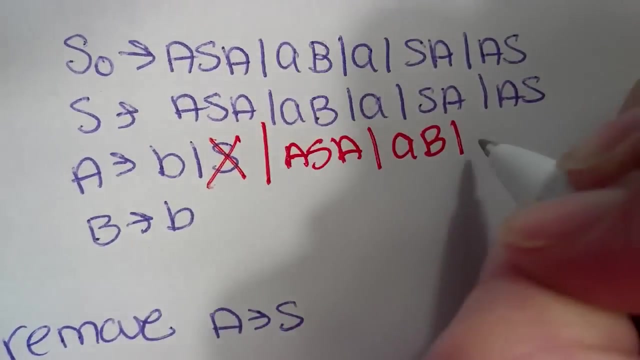 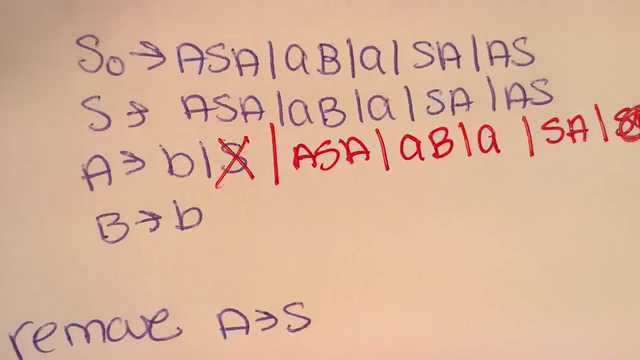 is to remove a points to s And again, just like when we knew what s not pointing to s meant all we have to do is cross off the s here and replace it with what's in s. So we just put asa or ab, or a or sa or as. So that is our new equation, which is now simplified. 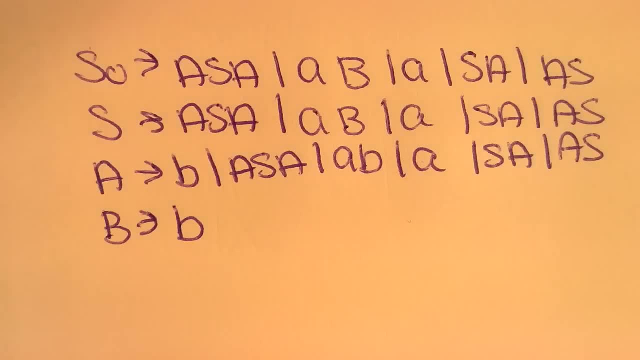 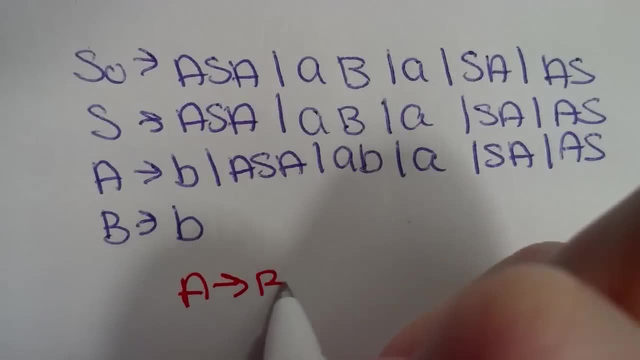 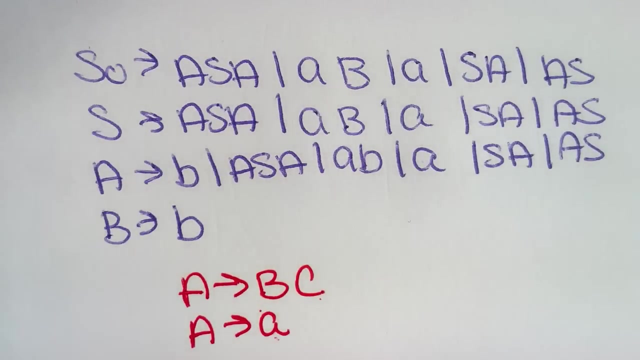 down here Now as a reminder, to be Chomsky Normal Form. we need to have this grammar in the form of a points to bc or a points to a, where b and c are our variables and a is our terminal, And there are just a few places where it does not hold. So if you look, 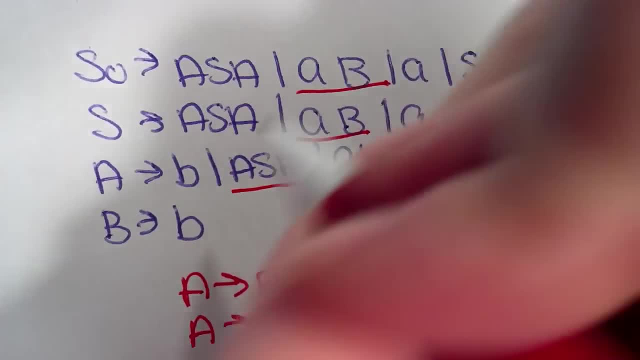 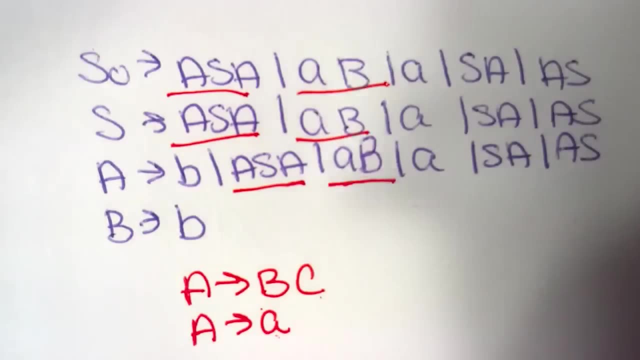 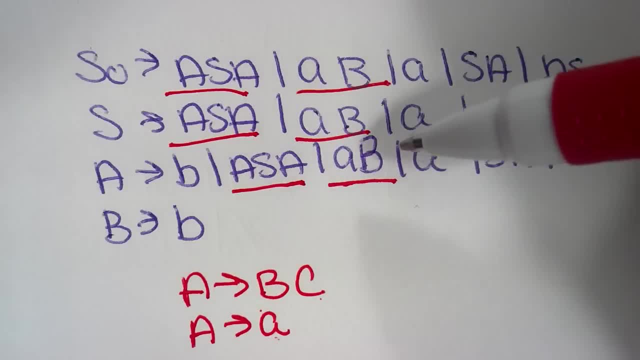 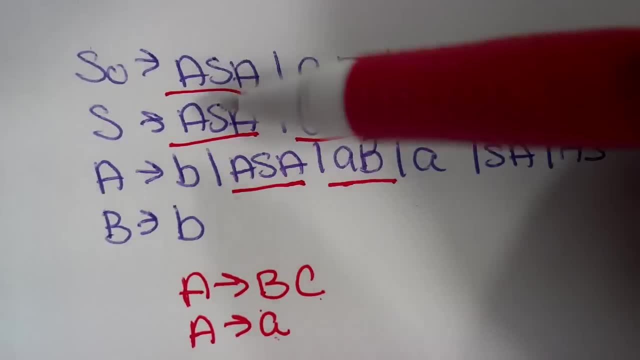 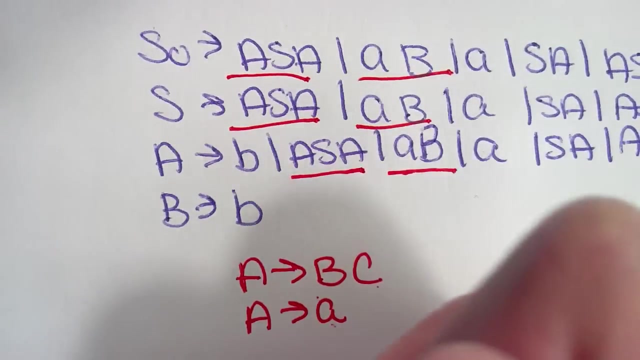 does not hold. So in order to make this Chomsky Normal Form, we have to create new variables to then replace the terminals or the variables. So, for example, what we're going to do is we're going to add a? u points to a, So we have a? u points to a, So we have a? u points. 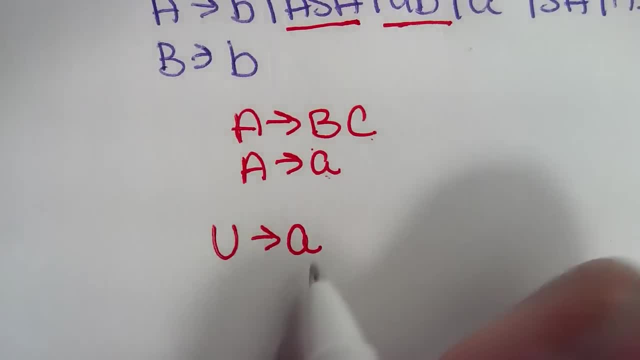 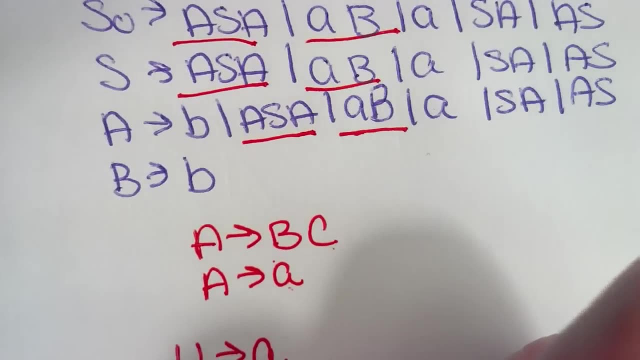 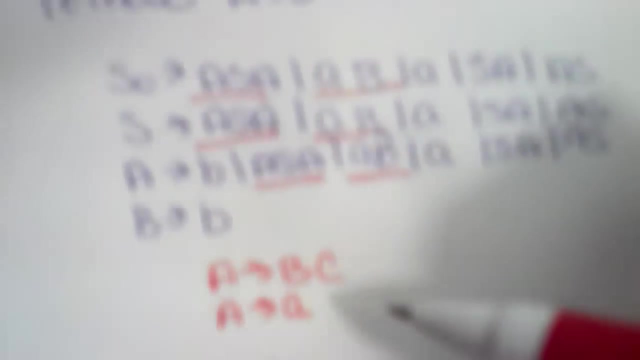 to a. So we have a new variable, u that's going to point to our terminal a, And we create a new variable, a1, that's going to point to our variables as. And what you do is you take these new variables and you replace them in our equation. So our new equation in the end, 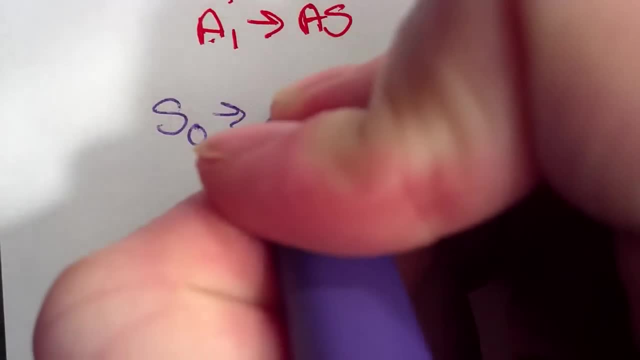 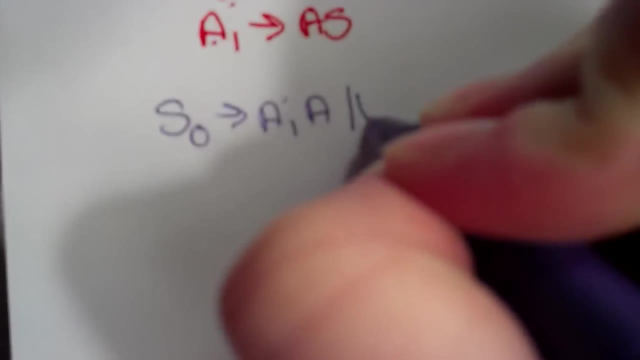 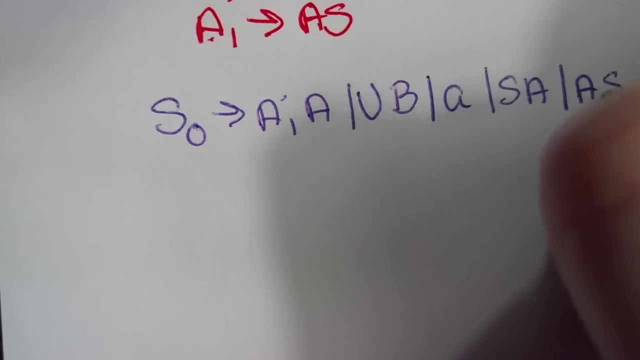 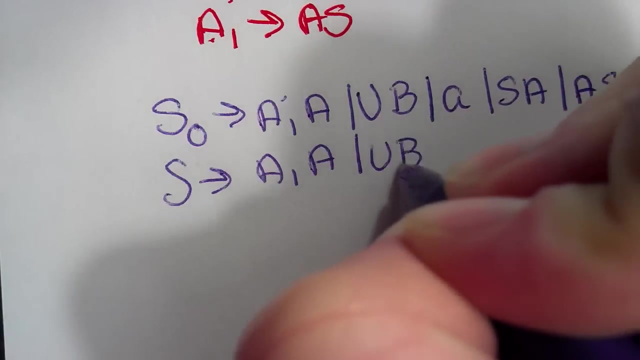 is going to be s naught points to a1. Subtitles by the Amaraorg community: A1, a or u, b, or a or s, a or a s And then s points to a1, a or u, b or.